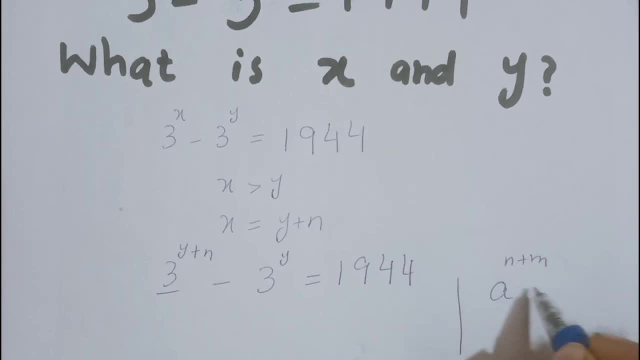 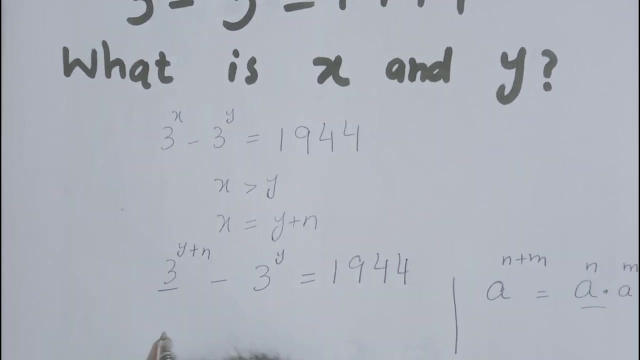 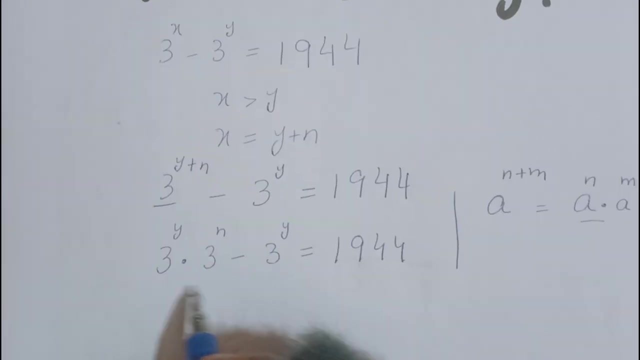 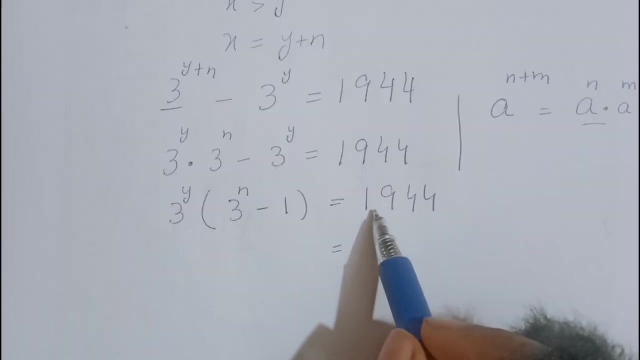 So let's try to solve this question. The question is: 3 raised to power x minus 3 raised to power y is equal to 1944.. What is the value of x and y in this question? So let's try to solve this question. The question is: 3 raised to power x minus 3 raised to power y is equal to 1944.. What is the value of x and y in this question? 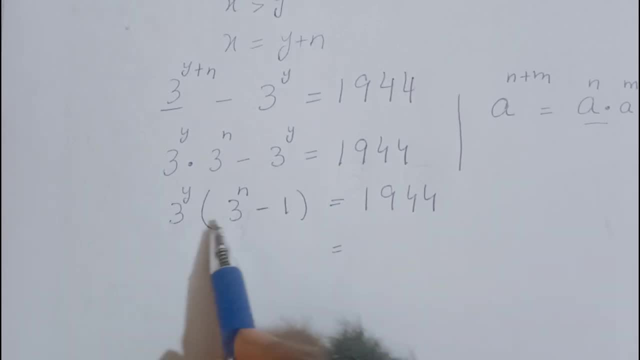 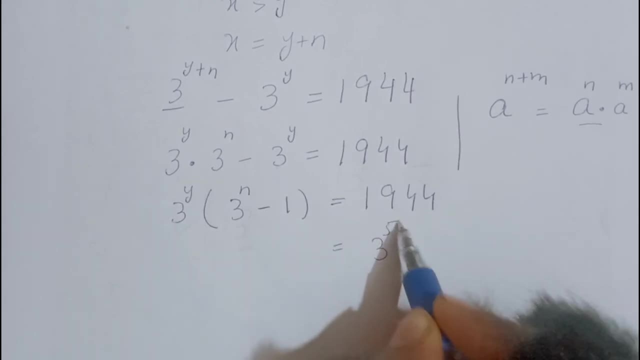 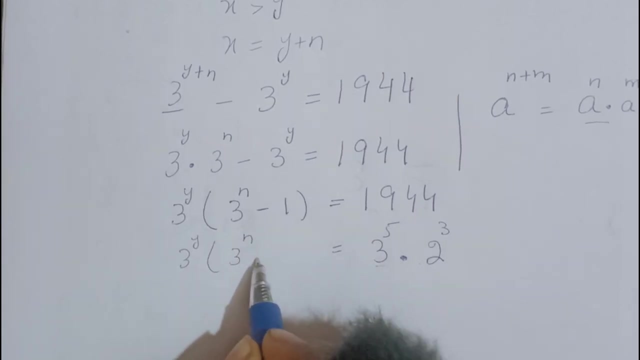 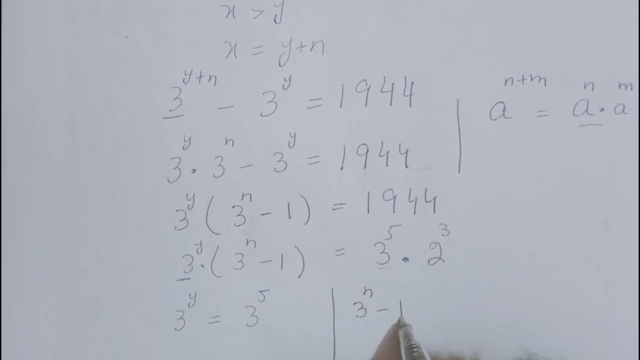 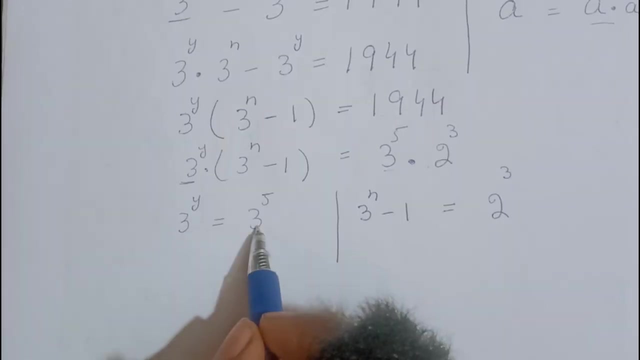 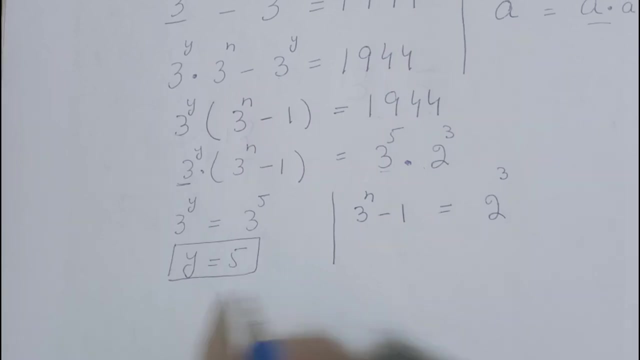 So let's try to solve this question. The question is: 3 raised to power x minus 3 raised to power y is equal to 1944.. What is the value of x and y in this question? So let's try to solve this question. The question is: 3 raised to power x minus 3 raised to power y is equal to 44.. What is the value of x and y in this question? 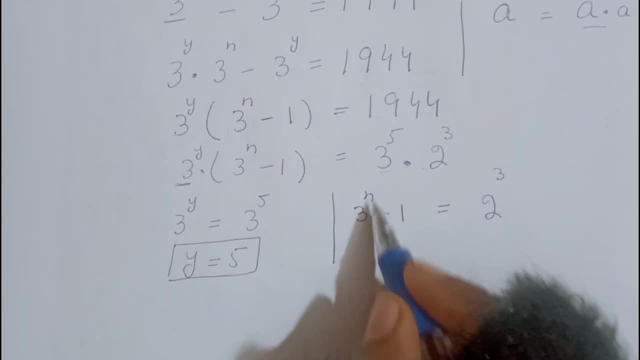 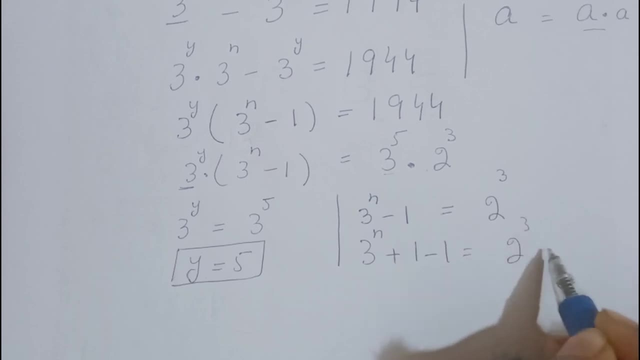 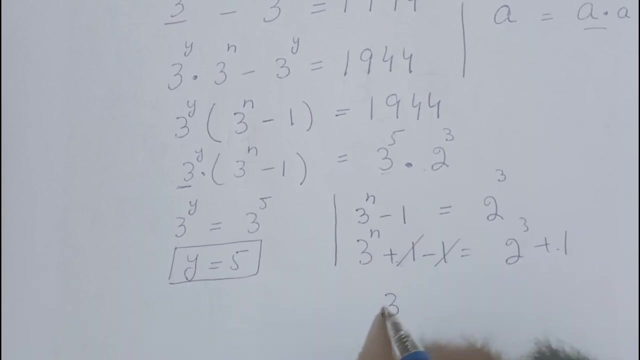 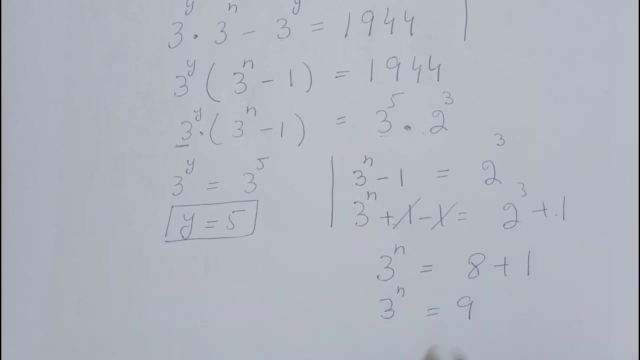 So let's try to solve this question. The question is: 3 raised to power x minus 3 raised to power y is equal to 44. What is the value of x and y in this question? So let's try to solve this question. The question is: 3 raised to power x minus 3 raised to power y is equal to 44. What is the value of x and y in this question?